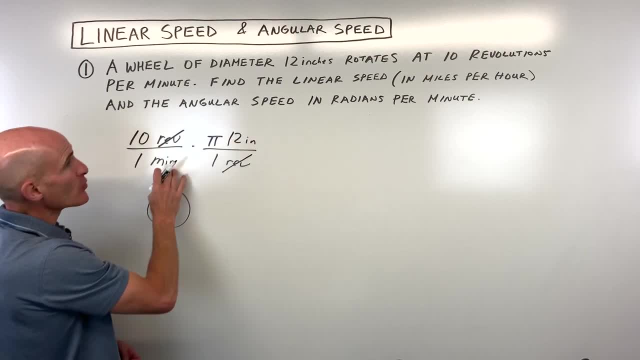 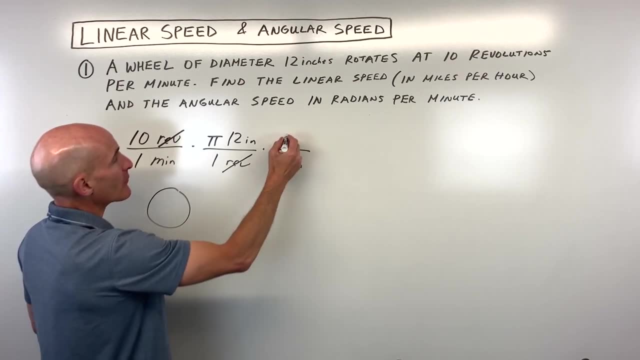 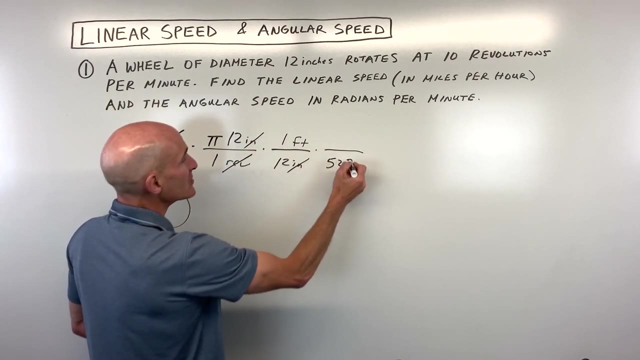 numerator and denominator. They cancel, and we have inches per minute. We want miles per hour. So let's go ahead and continue to convert this. We'll say there's 12 inches for every one foot, So you can see. the inches cancel numerator and denominator. and we know there's 5,280 feet for every one mile. So now you can see. 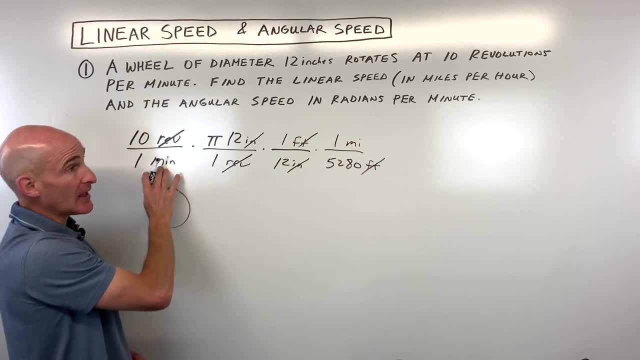 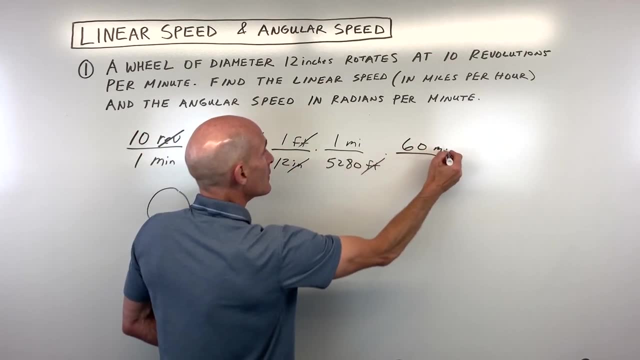 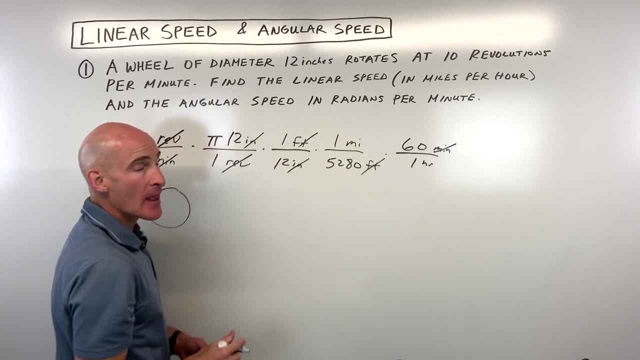 the feet are canceling and we have miles per minute. We want miles per hour, so we know that there are 60 minutes For every one hour. Now the minutes in the numerator cancel with the minutes in the denominator and we have miles per hour. So all we're going to do is we're going to multiply all these numerators together. 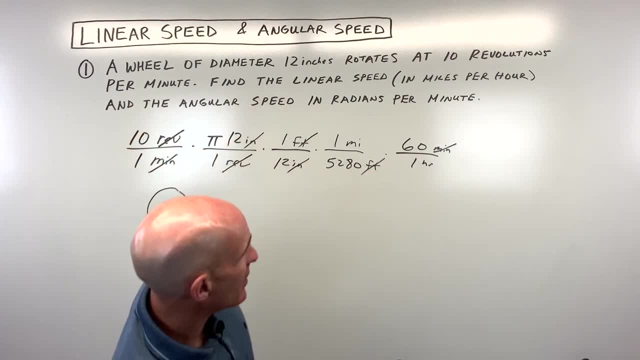 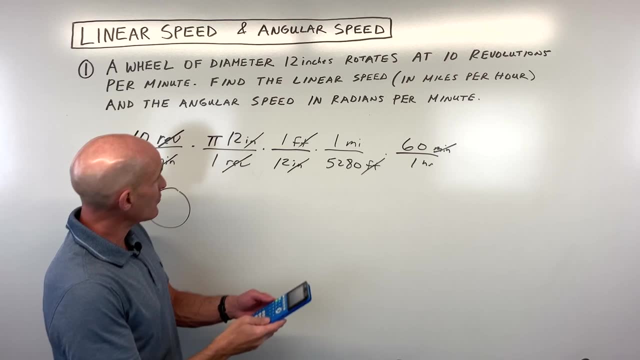 all these denominators together and then we're going to divide. So let's go to the calculator and do that, So that comes out to 10 times 12 times pi, You can do 3.14.. I'm using the pi key. 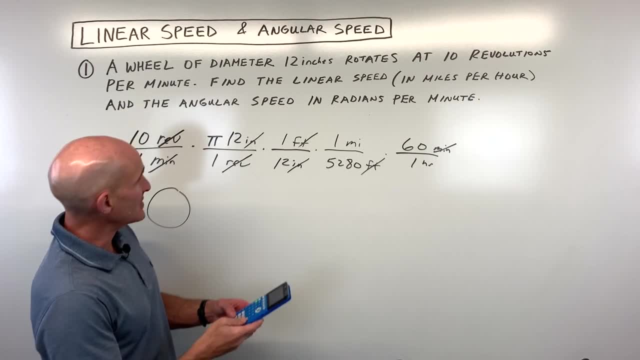 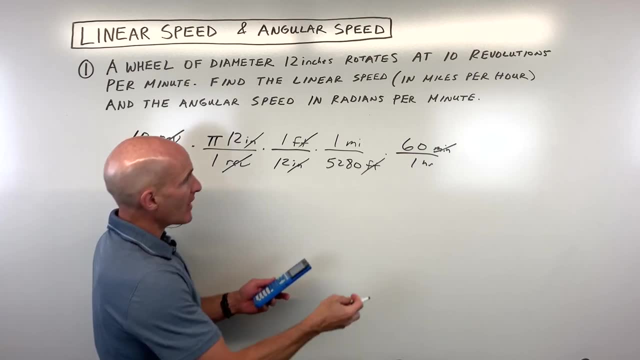 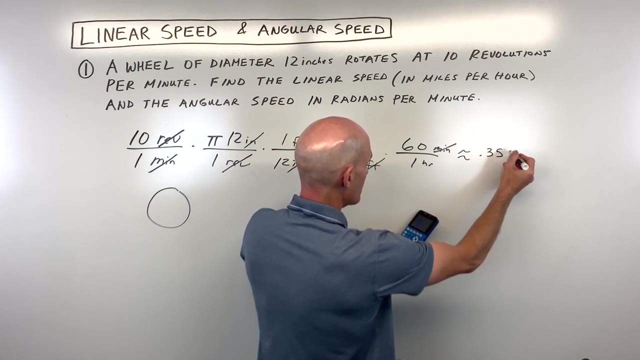 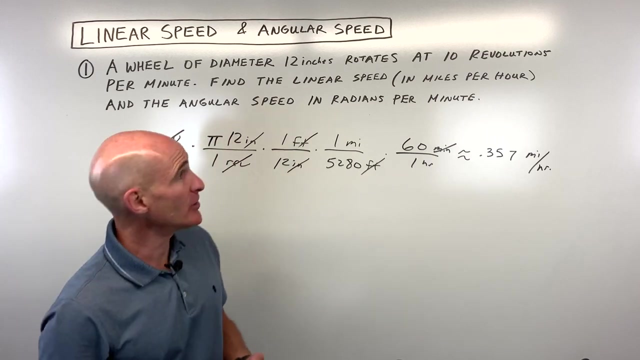 times 60, all divided by- in parentheses, 12 times 5,280.. So that comes out to approximately 0.35. actually let's do 0.357 miles per hour. Now let's say we want to do the angular speed. So that's the second part of the question. 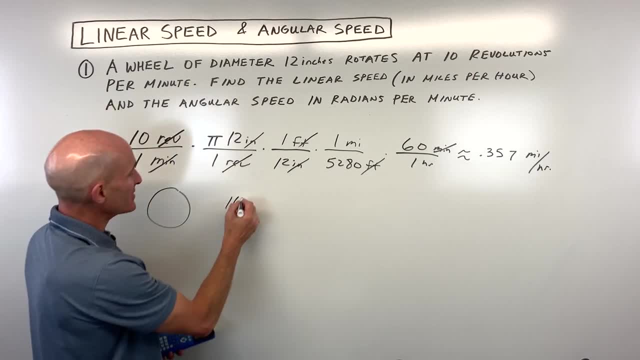 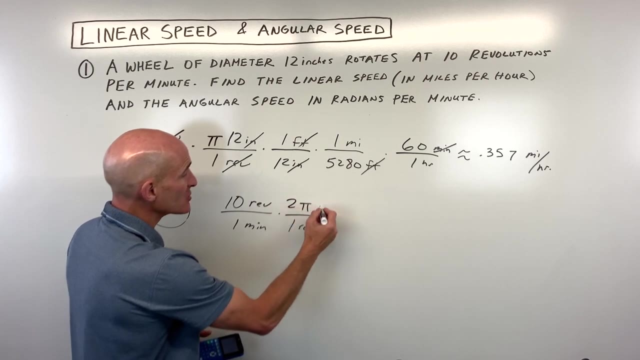 I would go back to the 10 revolutions per minute. So we'll say 10 revolutions per one minute. but we know that for every one revolution- see, it turns once around. that's 360 degrees, or that's the same as two pi radians. so you probably know that from your unit circle, so two pi radians per 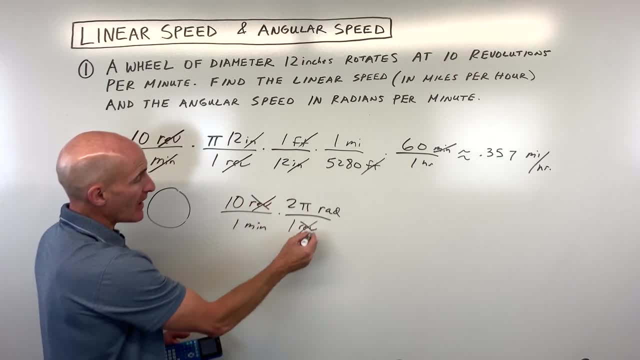 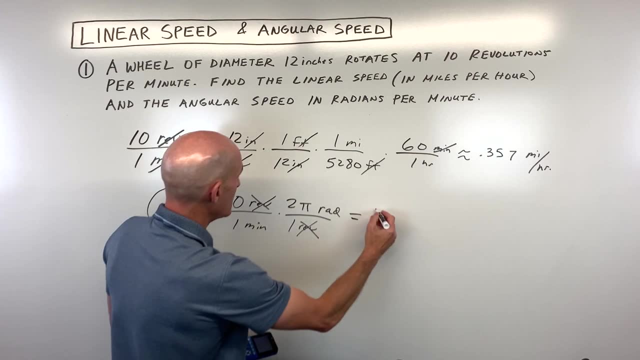 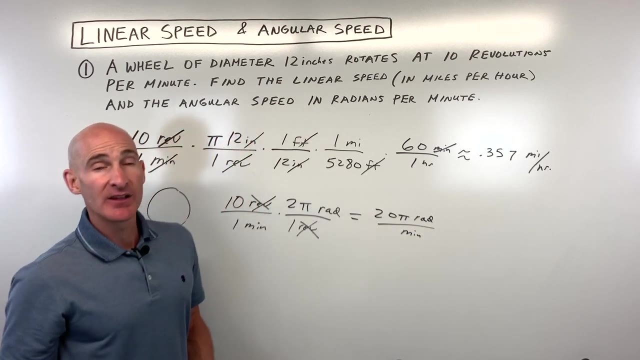 one rev. notice: the revolutions cancel numerator and denominator and we're left with radians per minute, and that's what we want. so if we go ahead and multiply horizontally here, we get 20 pi radians per minute. and you got it. let's take a look at another example. 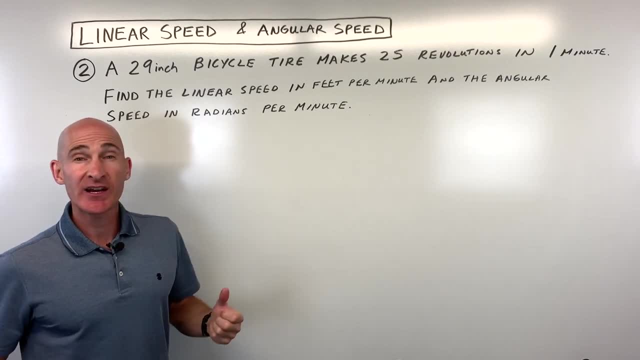 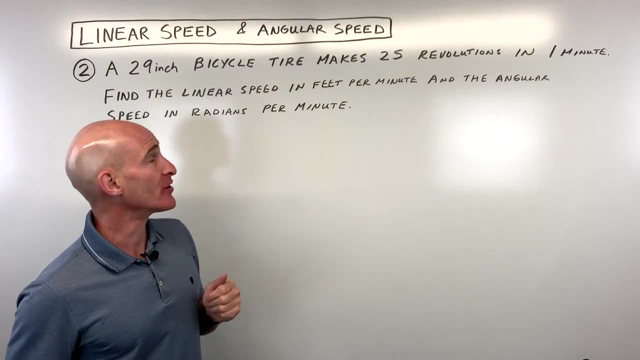 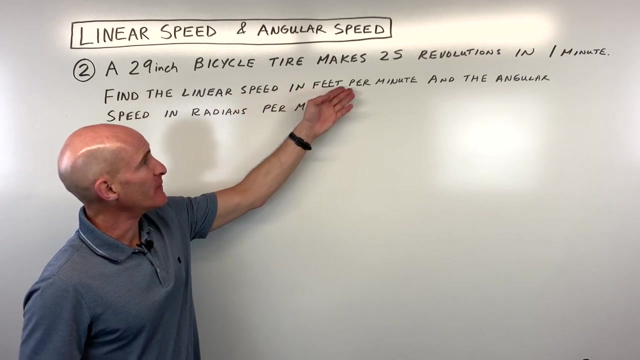 okay, see if you can challenge yourself and do the second problem on your own. we've got a 29 inch bicycle tire, and when they say 29 inches, that means the diameter of the tire is 29 inches. it makes 25 revolutions in one minute. what's the linear speed in feet per minute and the angular? 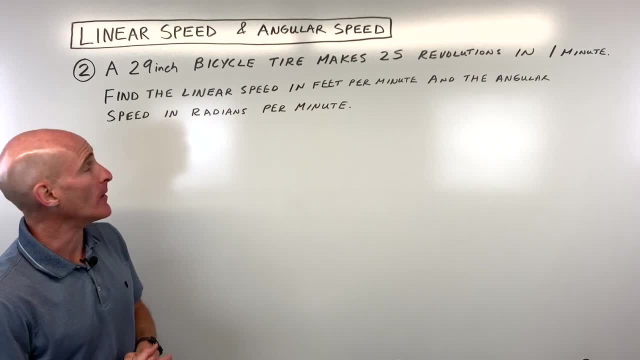 speed in radians per minute. so how would you go ahead and do that one? well, if i was going to do it, i would start off with the 25 revolutions in one minute. so 25 revolutions in one minute. and we know that for every one revolution once around, that when the tire makes one complete turn, it's going to travel 29 pi. 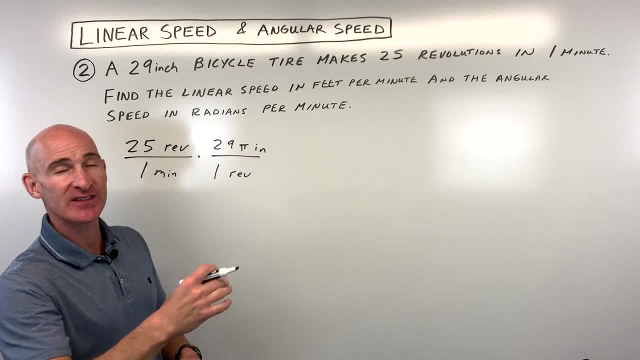 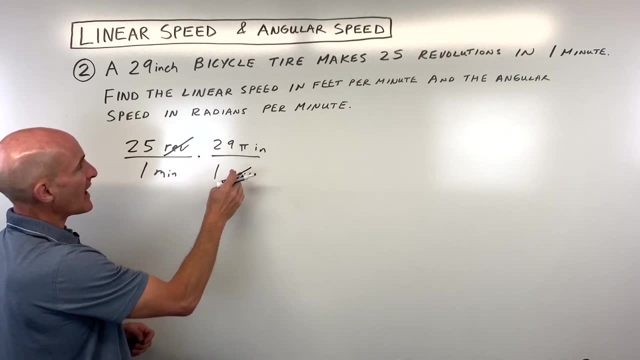 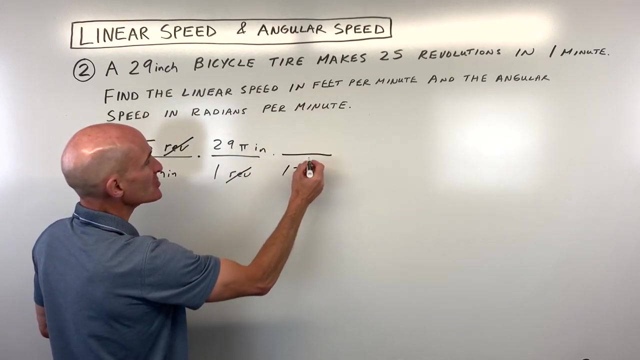 inches because, remember, pi times diameter is the circumference, that's the distance once around that bicycle tire. but notice, notice that when the tire makes one complete turn it's going to travel. now we're the revolutions are canceling numerator and denominator. we're left with inches per minute. we want feet per minute, so we're going to take it one step further for every 12 inches. 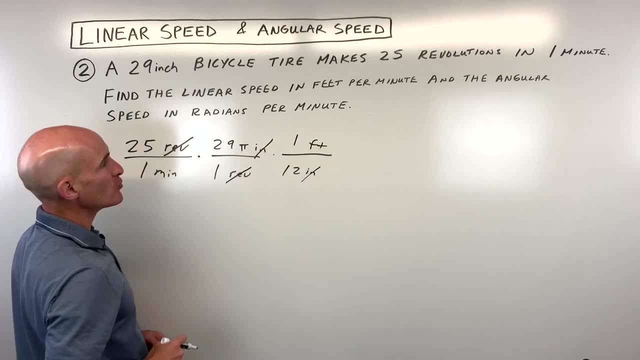 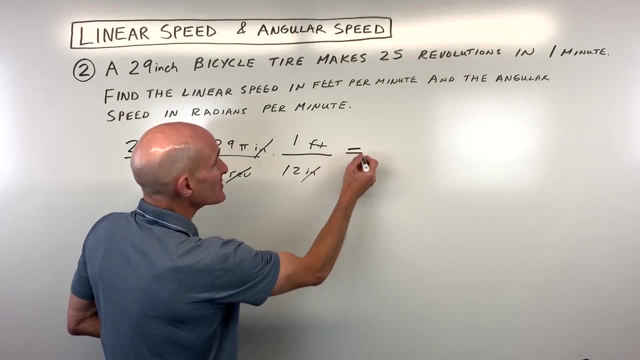 that's one foot, so you can see the inches are canceling numerator and denominator and we're left with the units feet per minute, which is what we want. now. sometimes your teacher will say: you know, leave this as an exact answer. and if that's the case, you would want to leave this pi in here. 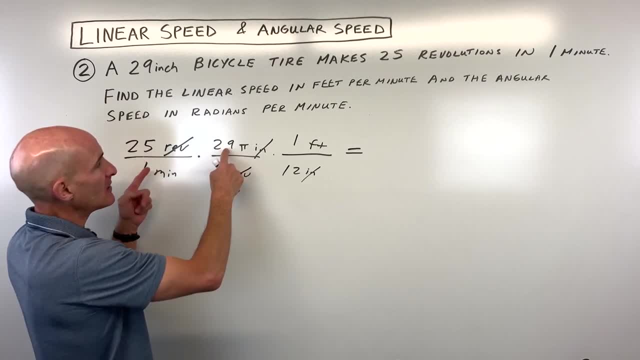 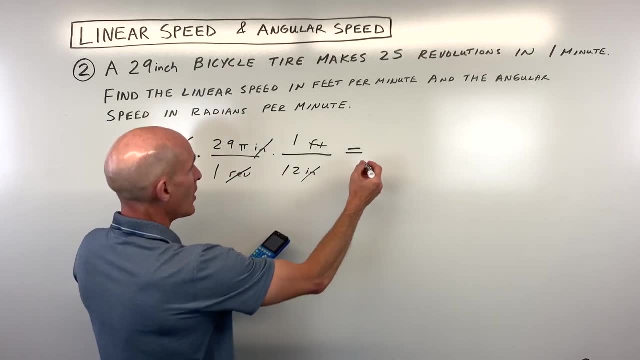 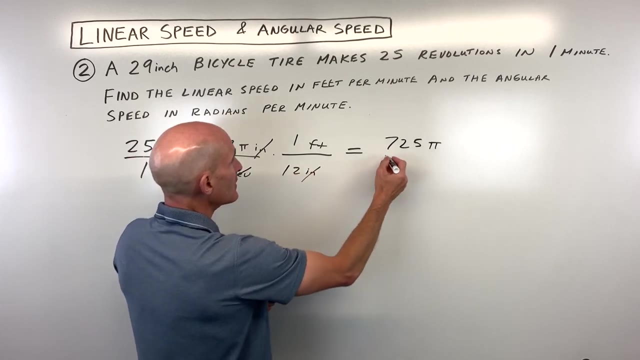 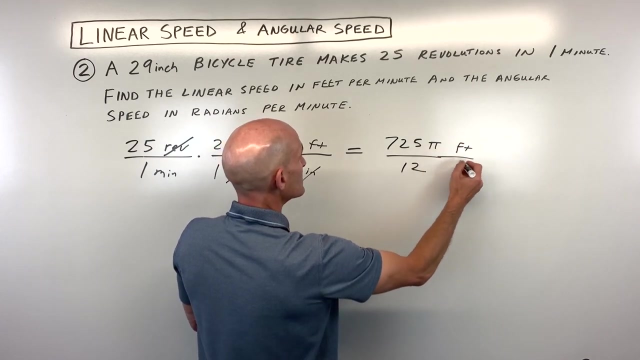 so we're just going to multiply 25 times 29 times one. so let's go ahead and do that one real quick on the calculator. let's see: so 25 times 29, that k times one is 725, pi. one times one times 12, it comes out to 12, and this is in feet per minute. okay, but now notice, you can reduce this. 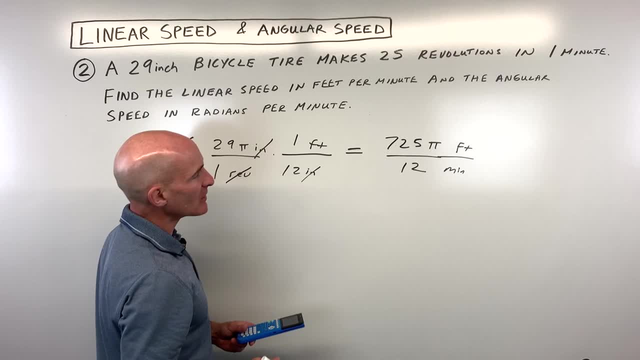 down a little bit. let's see. does that reduce down? let's see nine five. no, it doesn't look like it reduces. so this would be an exact answer: 725 pi times one. so we're going to do that real quick on the calculator. let's see. does that reduce down a little bit? so this would be an exact answer: 725 pi. 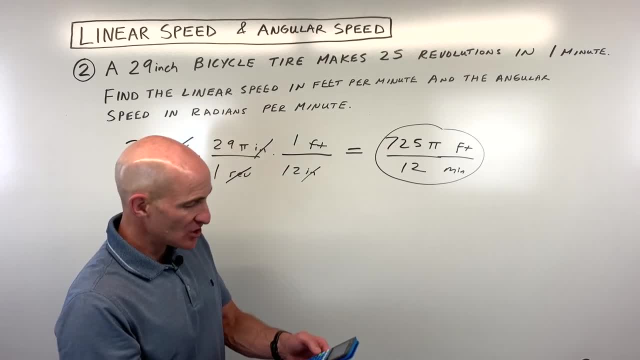 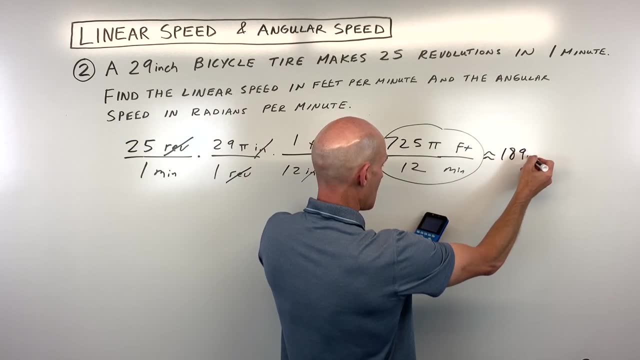 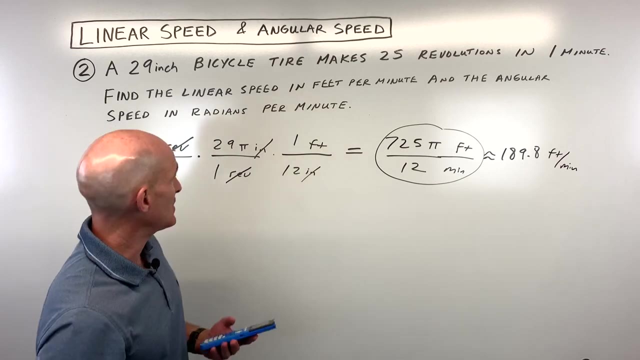 over 12 feet per minute. but if we want to get an approximation, i'm going to go ahead and use the pi key. it's approximately 189.8 feet per minute. now let's go ahead and do the angular speed. so the angular speed again, i like to go back to the revolutions per minute, the 25 revolutions per one.